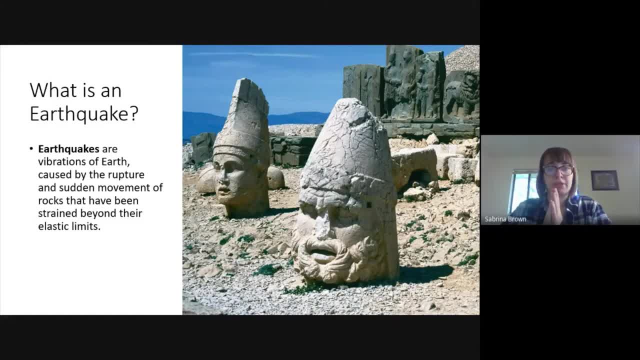 Remember back to our plates when we talked about plate tectonics and that those transform boundaries where those plates are slipping past each other. sometimes they get friction. that kind of prevents them from moving in. They can bend a little bit elastically. 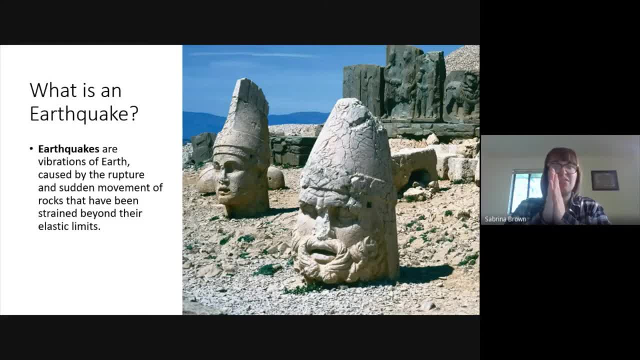 but then, once they're strained beyond those limits, right, they reach their limit and they can't bend anymore. that pressure, that friction gives way and then you have a slip or sudden movement along that fault and that causes the earth to vibrate. 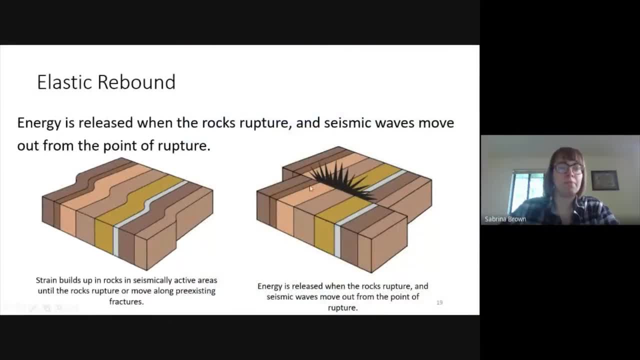 All right. so here's a picture of: we have movement along this little fault. it's bending, and then it reaches a point where it can no longer bend anymore and it breaks or ruptures instead, and that all of that energy released and that, you know, it's just a little bit of a. 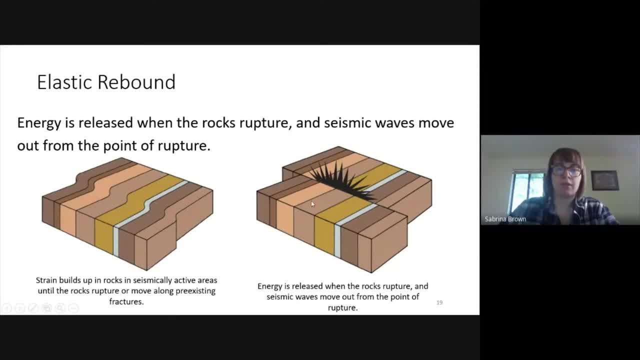 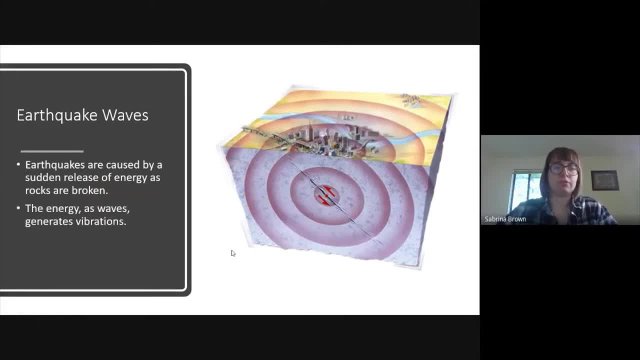 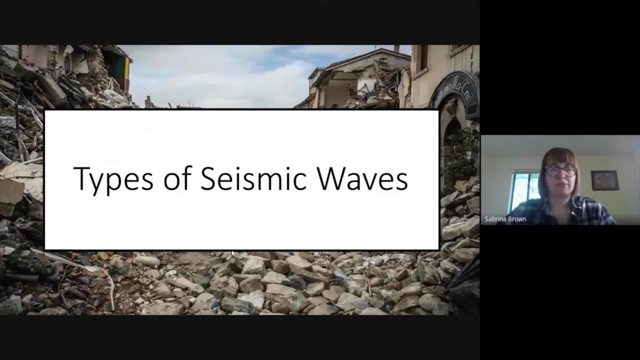 little bit of an energy release and that energy releasal is what creates an earthquake. So this energy release occurs as waves and those waves are what actually generate the vibrations of an earthquake. And we have four different types of seismic waves, so we can classify these earthquake waves which we call seismic waves. 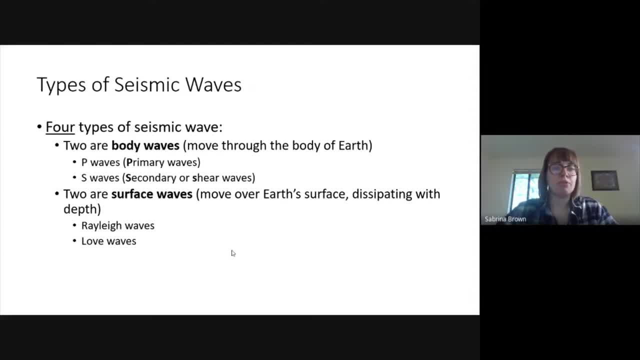 into two classes and four types. So two of the types of seismic waves are what we call body waves, and these waves move through the body of earth. One of those is a P wave, or primary wave, and the other body wave is an S wave, or a secondary wave. 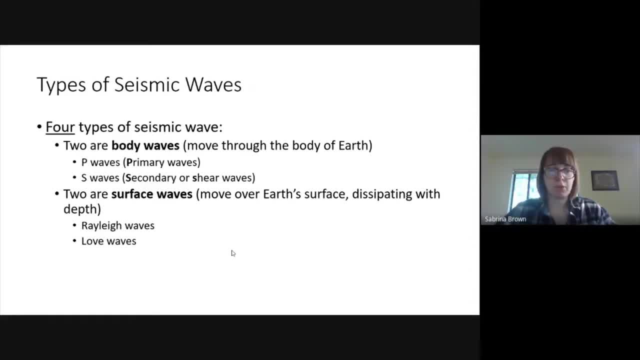 So our body waves are seismic waves. Earthquakes are seismic waves. Earthquakes are seismic waves- Earthquake waves that are moving through the body of earth- right, They're moving through the inside of earth. And then the other two types of seismic waves are what we call surface waves. 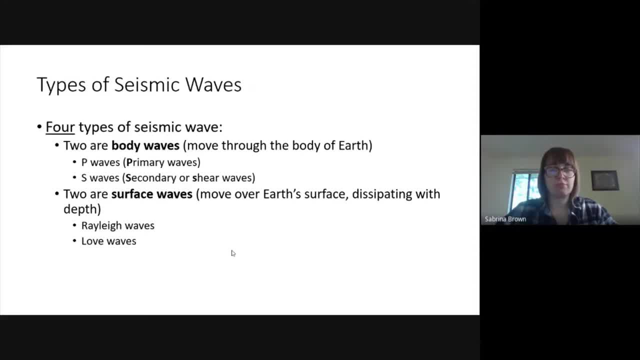 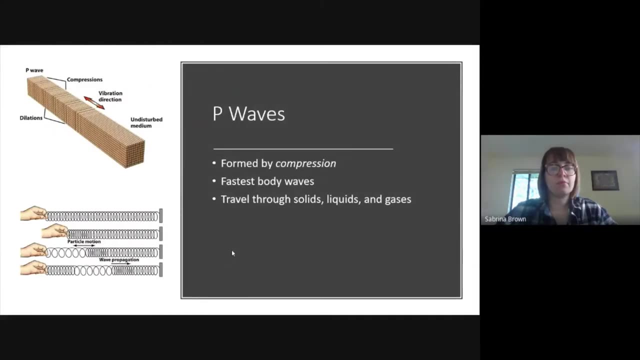 and surface waves move over the earth's surface right. They can't go through the inside of earth, They have to just move on the surface, And one of those are Rayleigh waves and the other are Love waves. So P waves are formed through the process of compression and these are the fastest body waves. 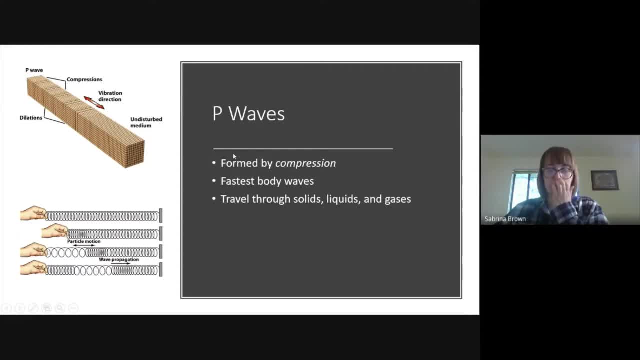 And P waves are able to travel through solids, liquids and gases So formed through compression, where you push motion, and then that motion moves on in the form of a wave. We will model each one of these types of waves in the lab to help you see what's happening. 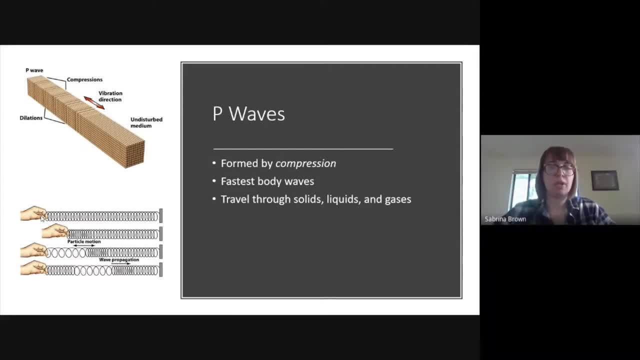 Okay, what this movement looks like. The important thing to know about P waves is that they can travel through solids, liquids and gases. S waves, which are our other type of body wave, are formed by sheer motion, So they're moved. they're formed by motion up and down instead of side to side. 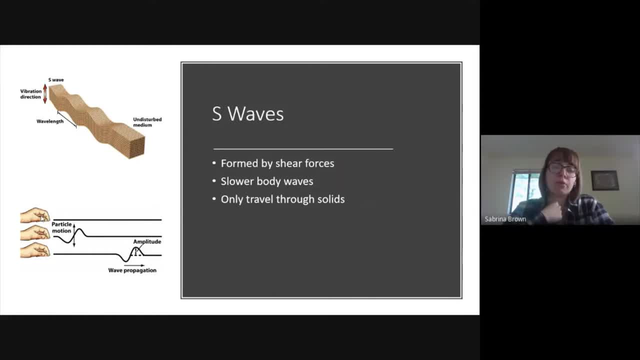 And these are the slower of the two body waves, And the important thing to know about S waves is that they can only travel through solids, right? So P waves, our primary waves, can travel through all states of matter. S waves can only travel through solids. 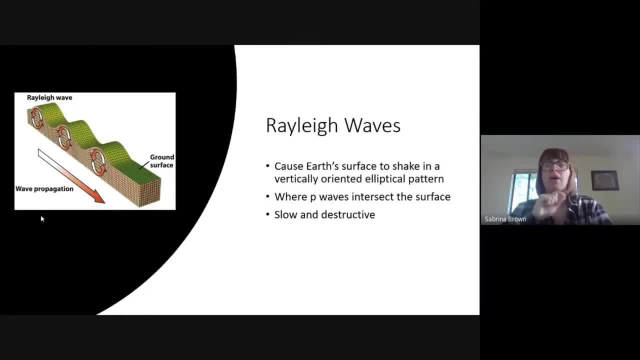 Reilly waves, our first surface wave, cause shaking in earthquakes in a vertically oriented elliptical pattern right. So they create these rolling waves, Sort of like the waves are generated in an ocean, And these occur where our P waves, our primary waves, intersect with the surface of Earth. 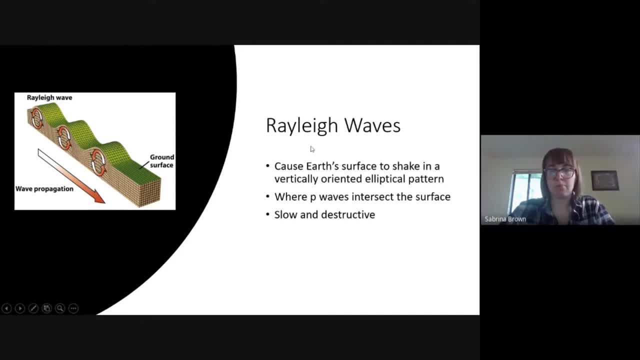 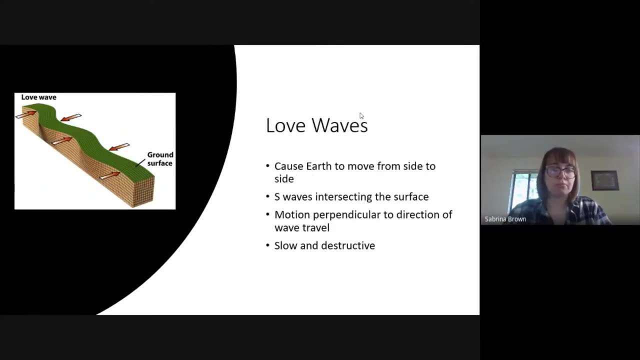 And they're very slow and destructive, right, Both of our surface waves are destructive because they're happening at the Earth's surface where humans are hanging out. So we see them as destructive because they're destroying a lot of our buildings and infrastructure. And then Love waves are waves that cause the Earth's surface to move from side to side. 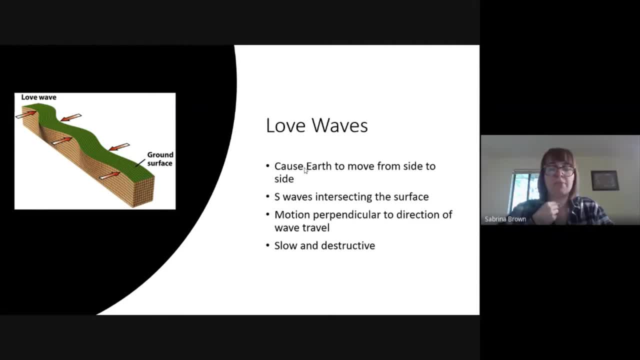 Sort of slithering like a snake, And this happens where S waves are intersecting at the surface, And so the motion of the wave is perpendicular to the direction that the waves are actually traveling Right. So the motion of Earth, the slithering motion, 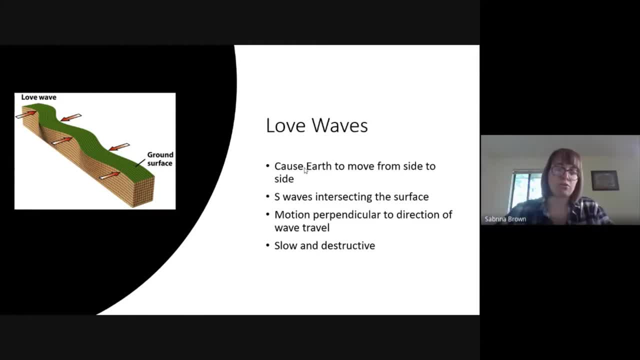 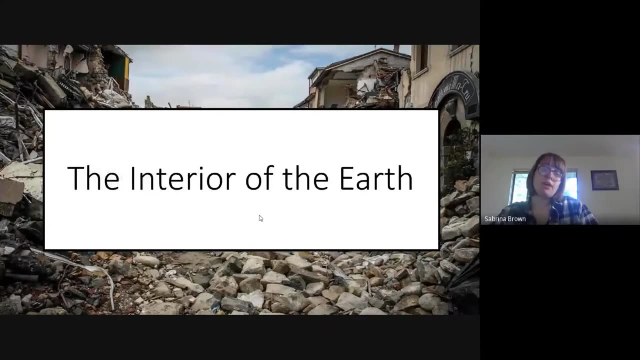 is perpendicular, perpendicular to the direction of the wave which is actually traveling this lengthwise. And again, love waves are surface waves, so they are slow and destructive. Alright, so the cool thing about earthquakes is that the way that earthquake waves travel, particularly primary and secondary waves, 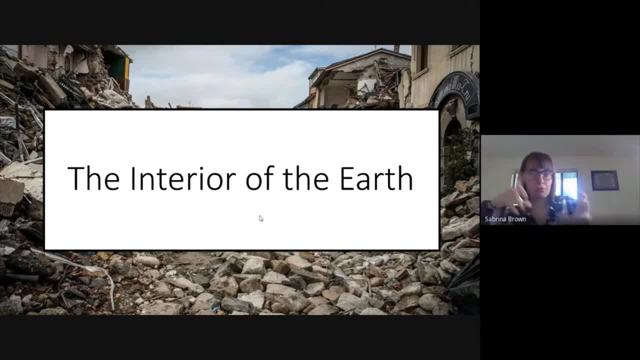 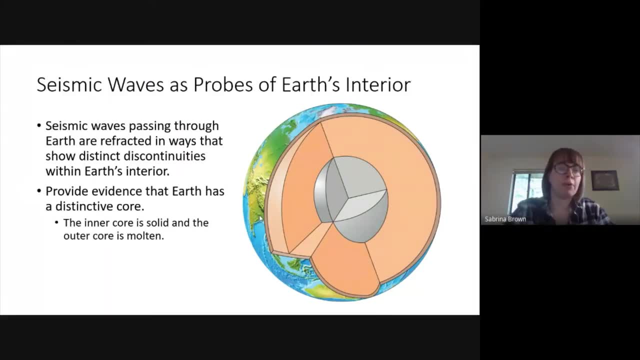 those waves that are traveling through the inside of Earth, through the body of Earth. they can tell us about what the inside of Earth looks like. So these seismic waves passing through Earth can be refracted, right diverted, in different ways that show that the Earth has distinct discontinuities or 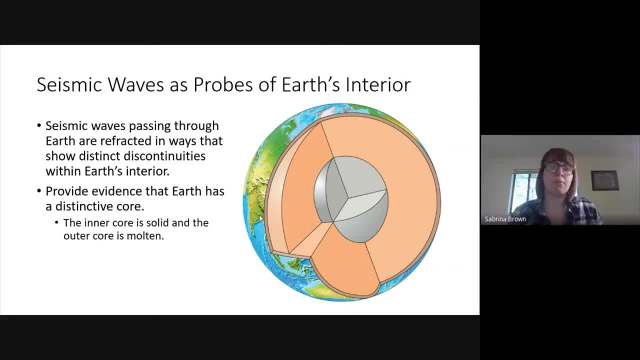 distinct differences inside of it. So this is how we know that Earth has a core. right, We've never been to the center of the Earth to see that it has a core, but we have inferred or we know that it has a core. So this is how we know that Earth has a. 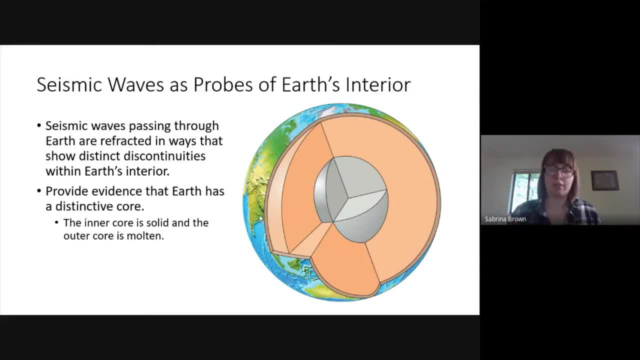 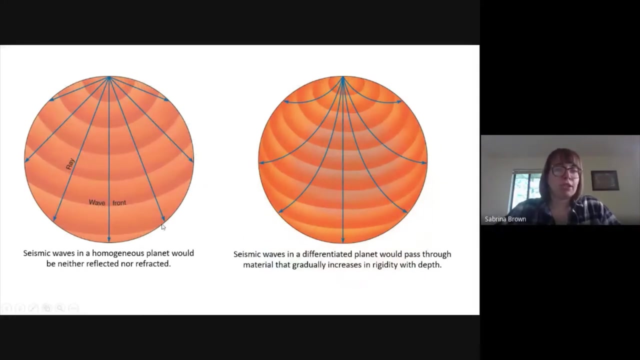 core and that the inner core is solid and the outer core is liquid, because we can understand these patterns of seismic waves passing through Earth to figure out that we have a differentiated planet. Alright, so if we didn't have a differentiated planet, all. 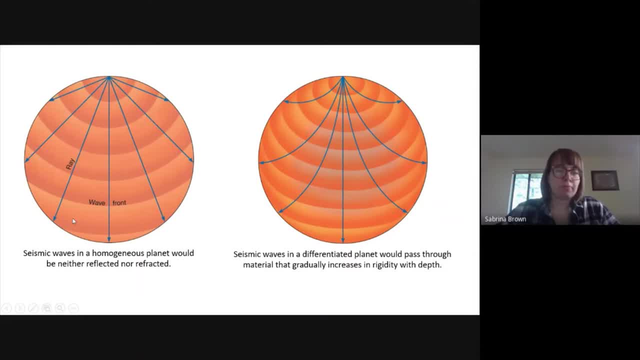 of the waves would just travel in straight lines through Earth. they wouldn't be reflected or refracted. But we have a differentiated planet, which means that those waves get bent or refracted as they pass through different materials, changing in structure, right how rigid they are, whether they're a liquid or a solid. 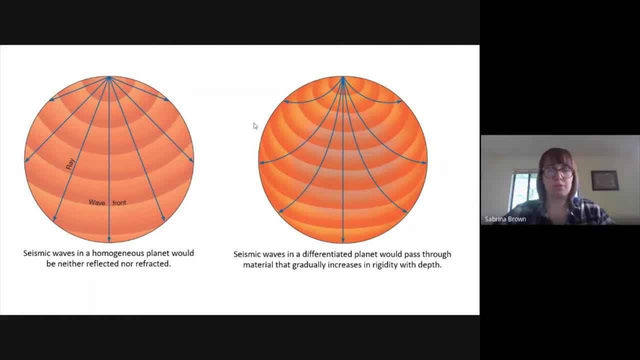 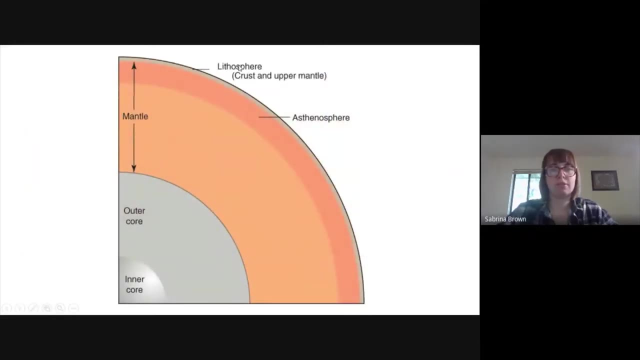 And so we can use these seismic wave deflections or refractions to understand the different layers of the inside of Earth. right? So remember, we have the lithosphere, which is the solid outer part, the asthenosphere, which is the plastic portion of the mantle that the lithosphere rides on. 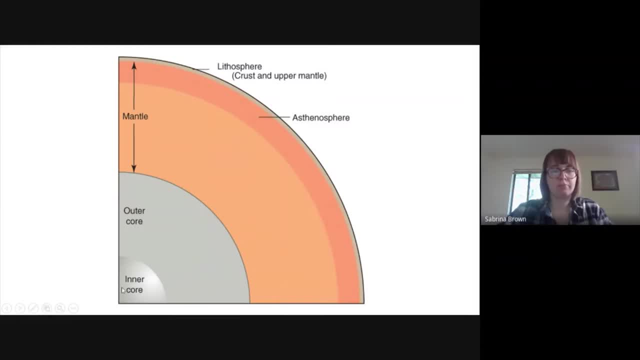 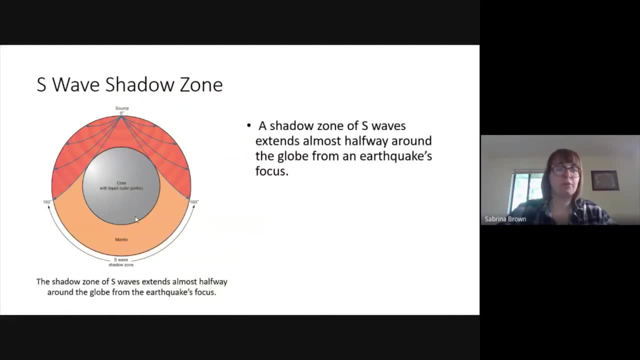 And then we have a liquid outer core and a solid inner core, And we know this with two pieces of evidence. One is that we have something called an S-wave shadow zone, And so if we have an earthquake here at zero degrees, scientists all over the world measuring these earthquake waves. 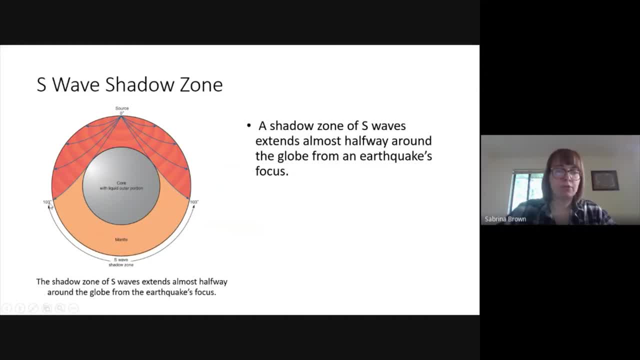 if you're on the other side of the Earth from where the earthquake occurs- from 103 degrees to 103 degrees away from that point source, your machines do not record any S-waves because you're in what's called the S-wave shadow zone. And this shadow zone 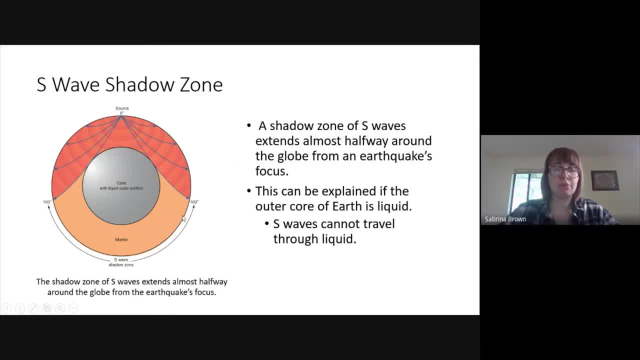 can only be explained if the outer core of Earth is liquid, and that's because our S-waves cannot travel through a liquid. So S-waves can't travel through a liquid, They can't travel through the liquid outer core, and so they hit the liquid outer core. 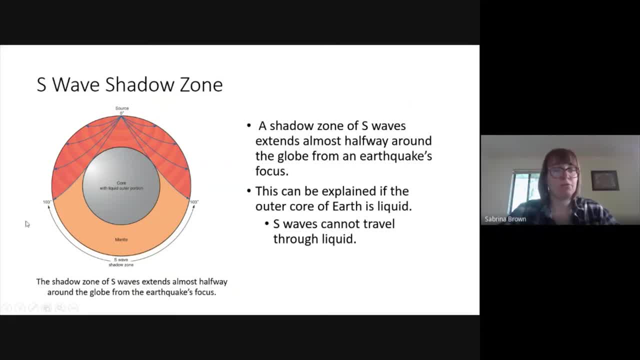 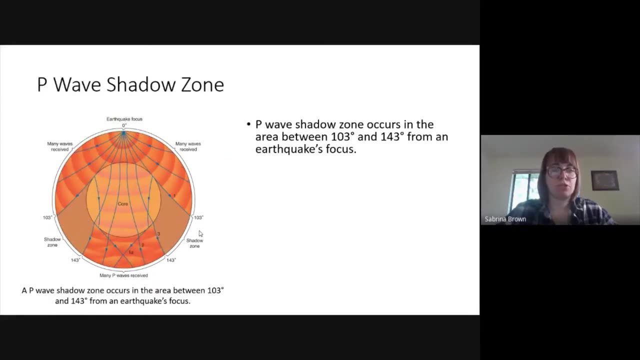 and then they can't travel anymore, They just stop. And so if you're on the opposite side of the Earth from an earthquake, you won't receive any S waves on your seismograph. and then the second piece of evidence for Earth's differentiation is from the P wave. 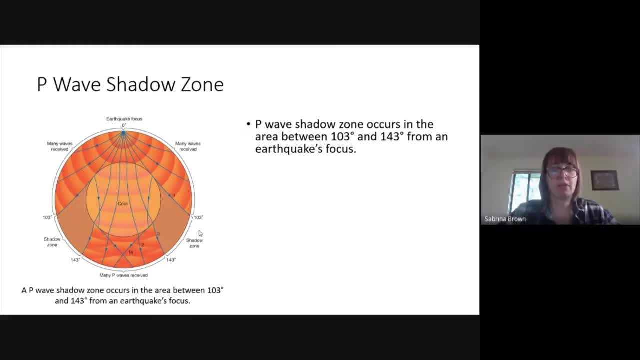 shadow zone. so our P waves, which are also body waves, also have a weird deflection happening in the in the center of Earth, where if you are between 103 and 143 degrees away from the earthquake, you will not receive any P waves, and this has to do with that. there's a solid central core through 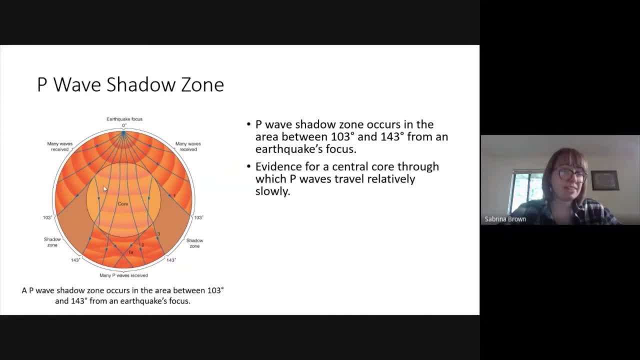 which P waves travel relatively slowly because it's very dense. so P waves can travel through the solid inner core. but because it's so dense they get slowed down and deflected And so you get this shadow zone right. so we get this complex pattern because there's lots of refraction happening inside of the earth to these P waves. but 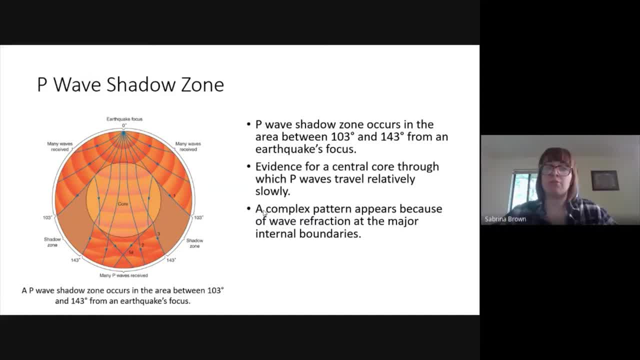 we can use our S wave shadow zone and our P wave shadow zone to infer that we have a solid inner core and a liquid outer core, and then how P wave velocity's change through a Earth's interior. we can calculate the density of the crust and the mantle as well, right So? 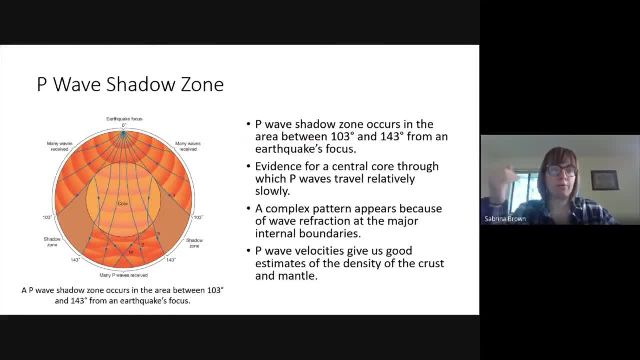 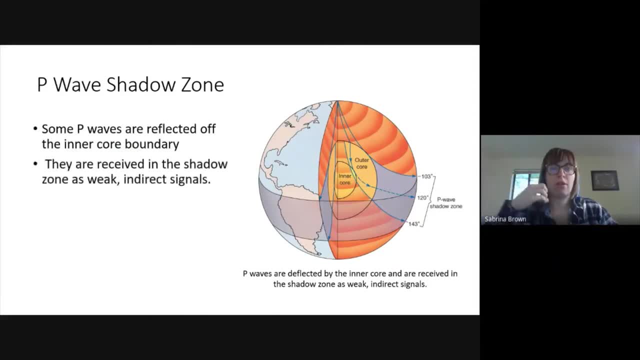 we can understand the core mantle and the crust from these seismic waves. So sometimes we do get P waves into the P wave shadow zone due to reflection off the inner core. but these are usually weak indirect signals. but again that's additional evidence for an inner core. 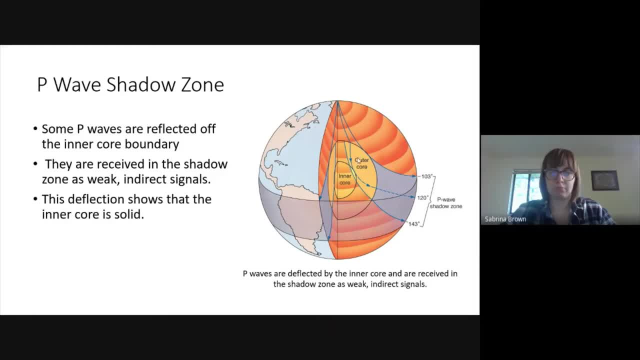 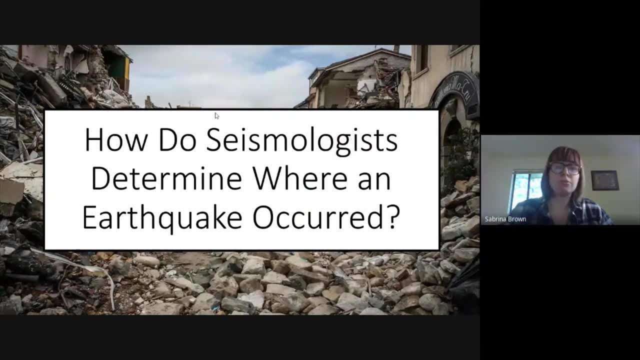 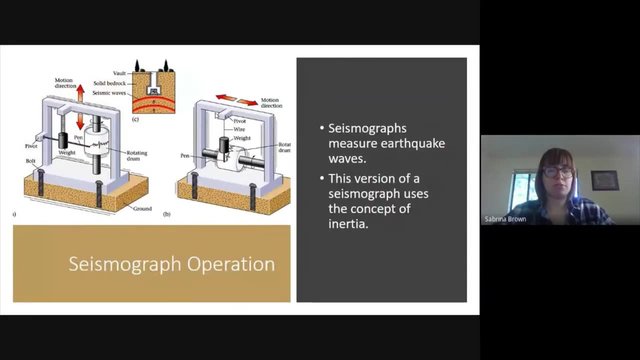 that is solid, Cool. So how do seismologists determine where an earthquake occurred? So seismologists- so seismologists are just scientists who study earthquakes- use a piece of data to determine where an earthquake occurred. So seismologists are just scientists who study earthquakes- use a piece of data to determine where an earthquake occurred. 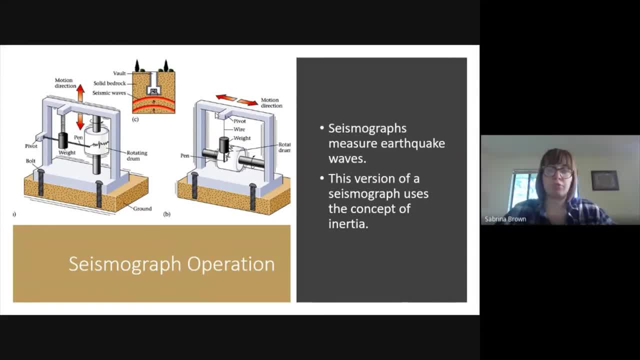 So seismologists are just scientists who study earthquakes, use a piece of equipment called a seismograph to measure earthquake waves. There's lots of different versions. Some of the older ones are based on the concept of inertia, where you have like a hanging weight and then a pen on paper. 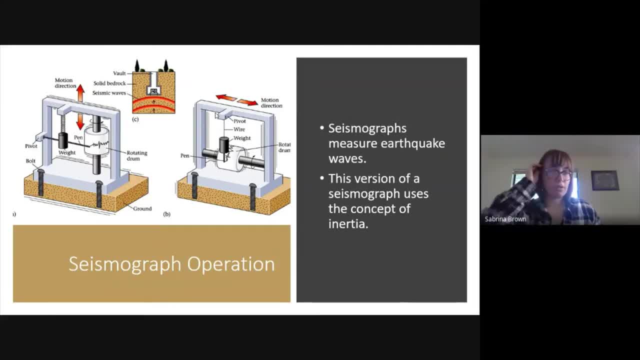 and as that weight moves with the motion of the earth, then it like writes a squiggly line on that paper. You might sometimes see these even like in museums, like if there's delicate stuff they put Graphic seismographs near delicate things, like in art museums. 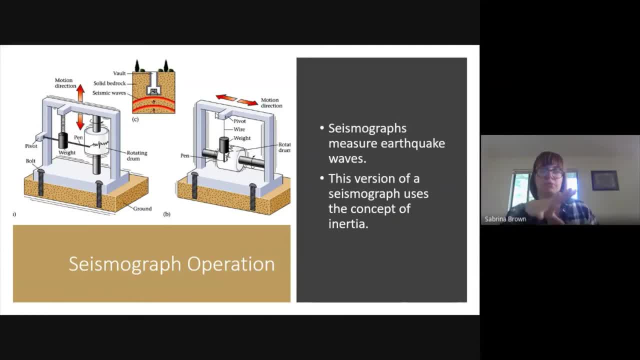 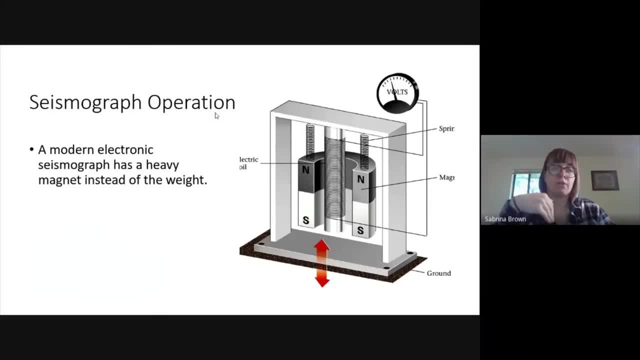 or in natural history museums to make sure that you are not causing too much disturbance to those artifacts. More modern seismographs are based on magnets instead of using, like this, inertia weight, but it makes a similar recording. A lot of seismograms, which are what the recordings we have of Earth's shaking are based on these squiggly lines from those older models. 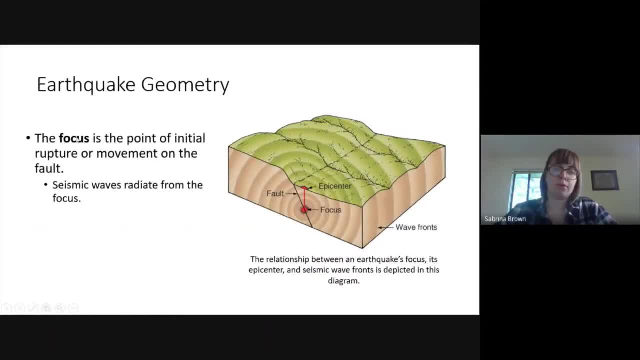 All right. so some vocab words you need to know about earthquakes are that the focus of an earthquake is the initial point of rupture, of movement along the fault. So usually this is deep within the Earth, along a boundary where two plates are moving next to each other. 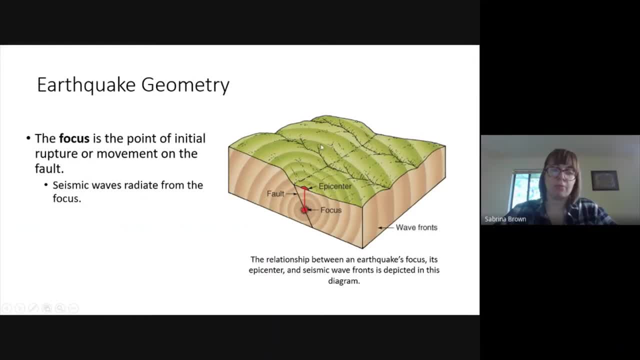 And then the seismic waves are radiating away from this focus. But the epicenter, which is usually the word you hear more often in the news when people are talking about earthquakes, is the point on Earth's surface directly above the focus, right. 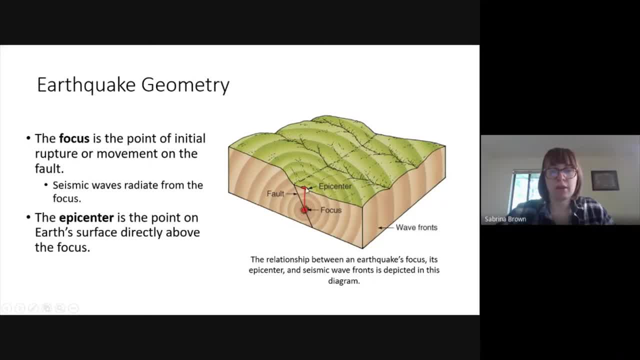 So epicenter is the point on the Earth's surface, directly on top, So it's directly above the focus or directly above the focus. And we care about the epicenter because it's the place on Earth that we can pinpoint geographically and say this is where the earthquake occurred below. 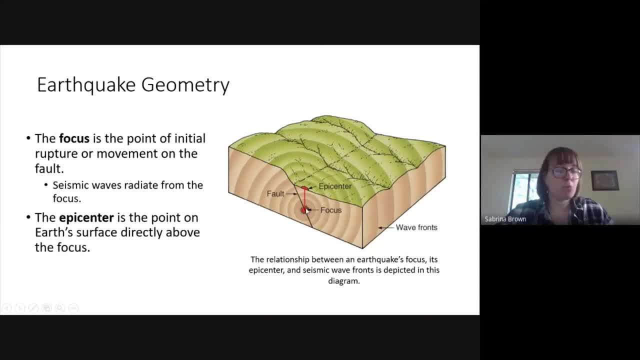 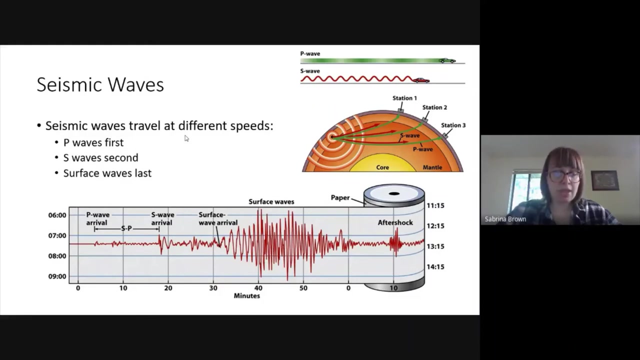 And it's the closest possible point to the focus, so it's going to be the place that has the most intense wave action from that earthquake. All right, so remember that seismic waves travel at different speeds and P waves are the fastest. So down here we have our seismograph right. 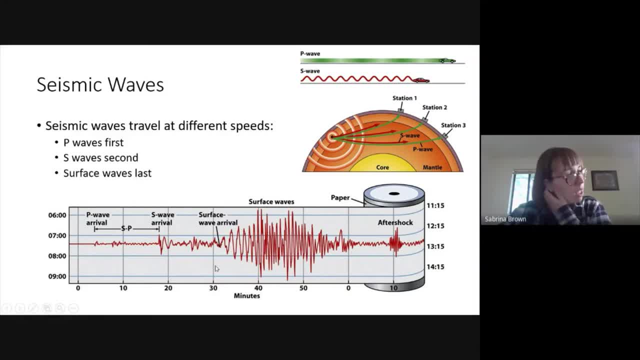 These squiggly lines are showing how much the Earth is moving, And our P waves always arrive first, right, So we have no movement. and then our first sign of movement is our P wave down here, And S waves arrive second, But they usually have a little bit of a higher amplitude. 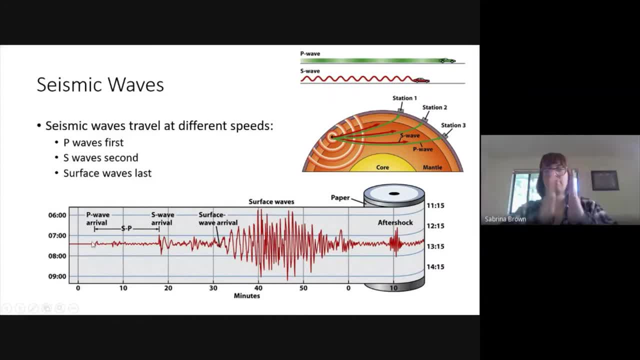 They're usually a little stronger than P waves, right? Because instead of this motion, accordion, motion of P waves, we have this motion of S waves, So they're a little stronger, causing a little bit more movement. right Up here we have our P wave moving through compression, our S wave squiggling along. 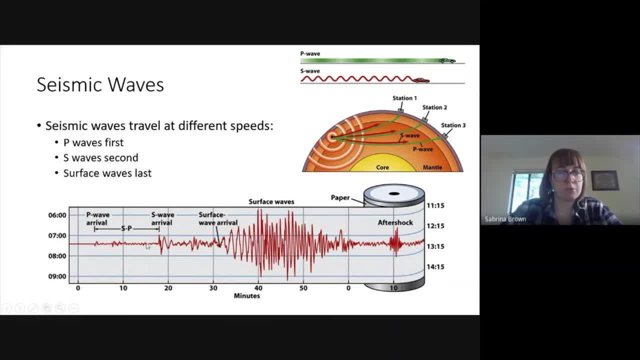 So our P wave arrives first, and then there's a period where we just receive P waves. So we have our P waves on our seismograph and then our S wave arrives. It's a little stronger, right? So those are our two body waves. 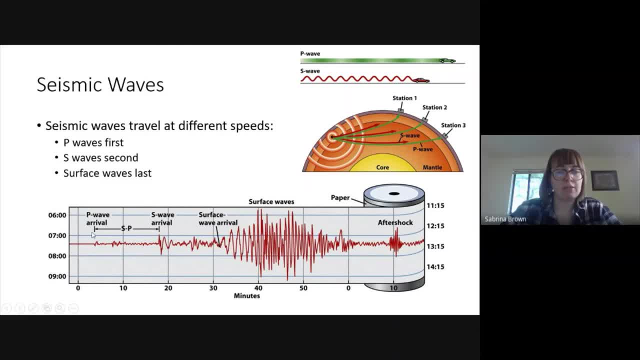 And then the difference in time between when the P wave and the S wave arrives is called the SP interval, And then for a while we have to wait, and then our surface waves are going to arrive last, But they have the highest amplitude because they are shaking the surface right where your seismogram is sitting. 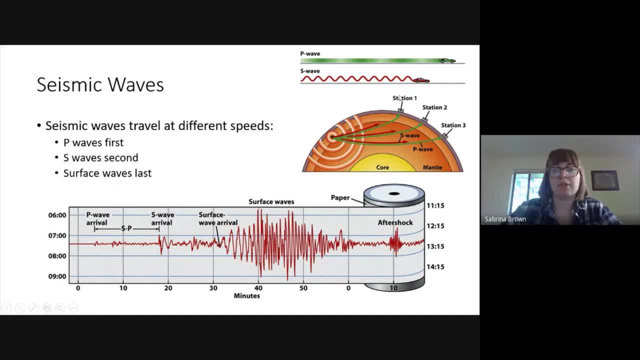 And then, depending on where your seismogram is- whether you're at station 1,, 2, or 3, these timings are going to be different. right, The closer you are to the epicenter or focus of the earthquake, the shorter amount of time you're going to have between the actual rupture at the focus and the arrival of your P and S waves. 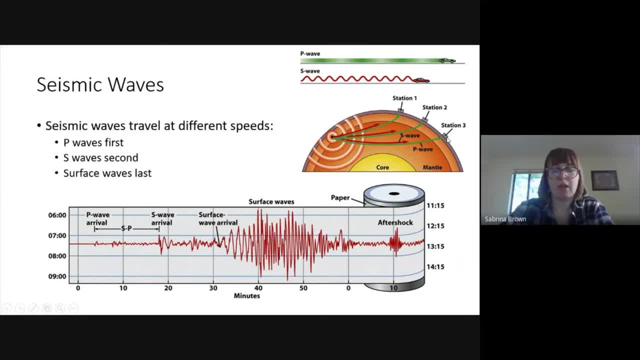 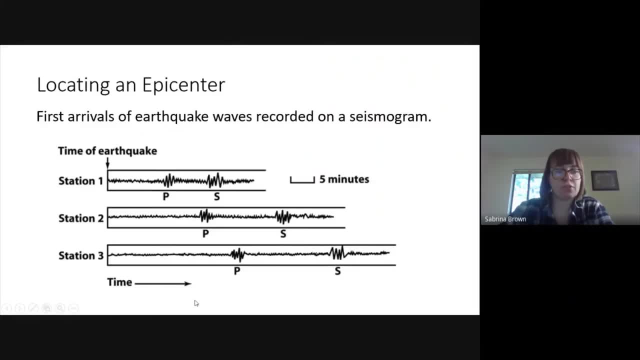 Okay. So the longer you are, the longer it will take the waves to get there and the longer interval between them you will have All right. So here we have three stations with earthquake waves, particularly our P and S waves. So you can see, station 1 is closest right. 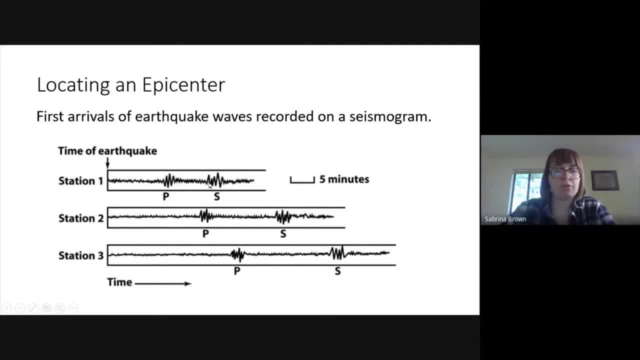 So our P wave arrives and then we have a relatively close, So we have a relatively short P to S time before our S wave arrives. And as we move farther away- station 2 is a little farther away. P takes longer to get there. 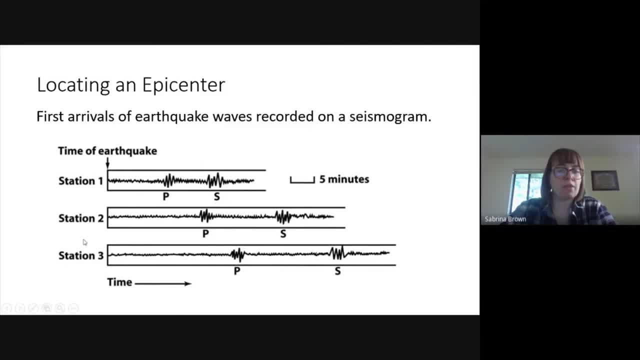 This interval between the P and the S wave is longer. And then the farthest station away, station 3,. our P wave takes really long to get there And then we have a long interval until our S wave gets there. So the closer you are to the focus of the earthquake, the closer together your P and S waves will be. 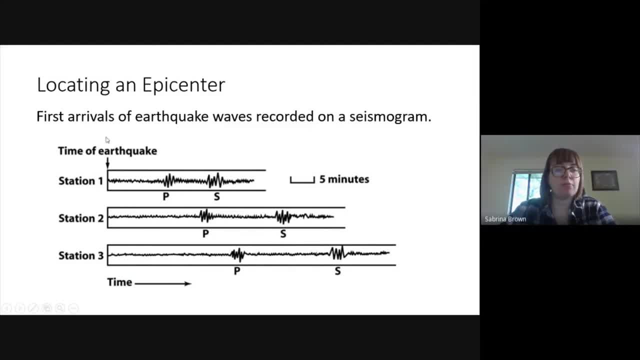 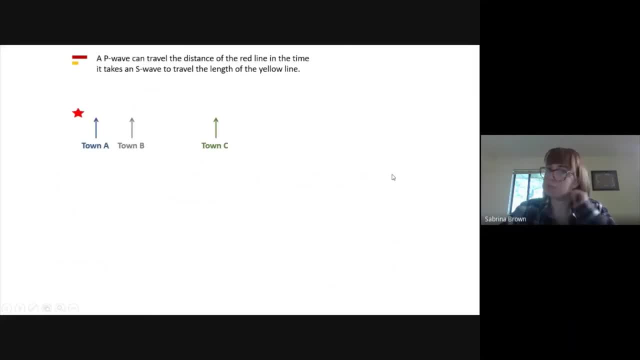 And the less amount of time you have to wait from the initial time of the earthquake for those waves to arrive at your location. All right, So remember, P waves move faster. So a P wave can travel the distance of the red line in the time it takes an S wave to travel the length of the yellow line. 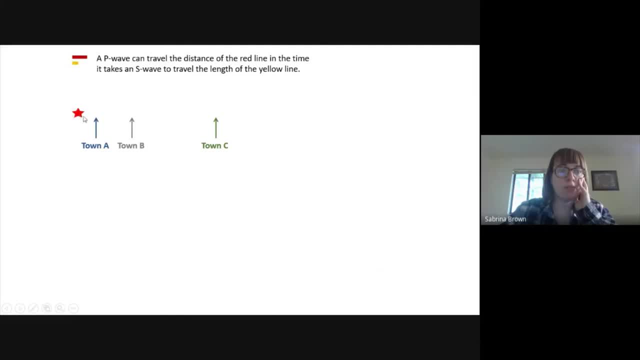 So P wave is traveling almost twice as far. Here we have our earthquake At the star, And then we have count A, B and C where we have a seismograph for each there. So our earthquake happens, And then we have waves traveling away from our earthquake. 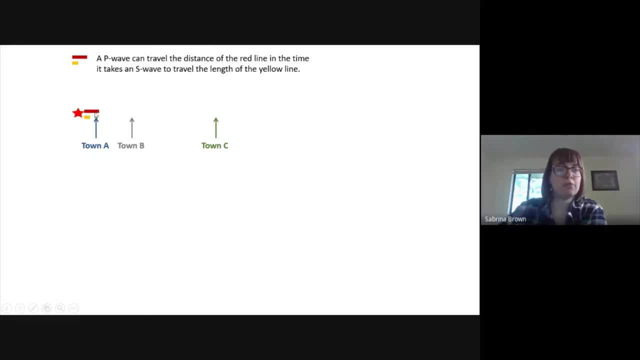 P waves are traveling faster than S waves, So here at time 1, sorry, I'll go back 1. We have, our P wave has traveled this far in the amount of time And our S wave has traveled this far. Our P wave arrives at town A. 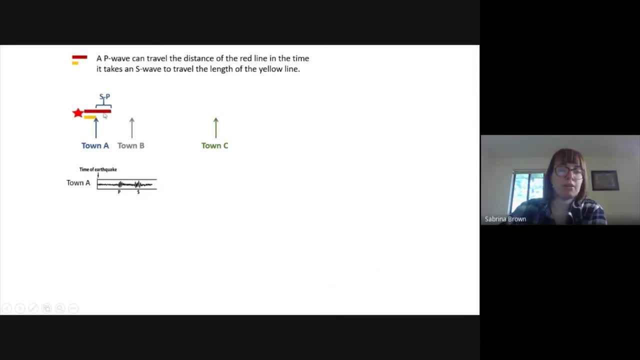 And then our S wave arrives at town A later. So here's our P wave arrival, and then our S wave arrival, And then, if we keep going, we see: okay, here's where our P wave has arrived. at town B: Our S wave's not there yet. 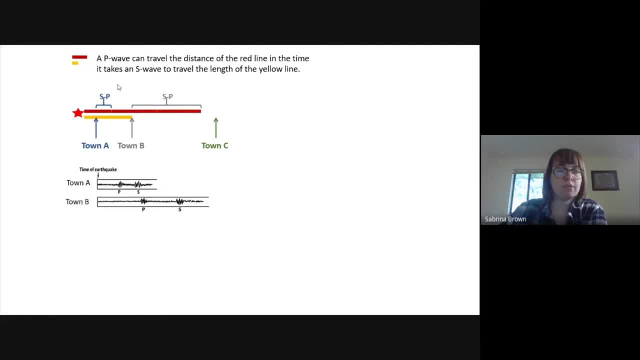 Keep going Until now, Our S wave has finally arrived. The P waves traveled that much farther already, Even though they started at the same place. So we have this longer interval before our P wave And we have a long S-P interval before our S wave arrives. 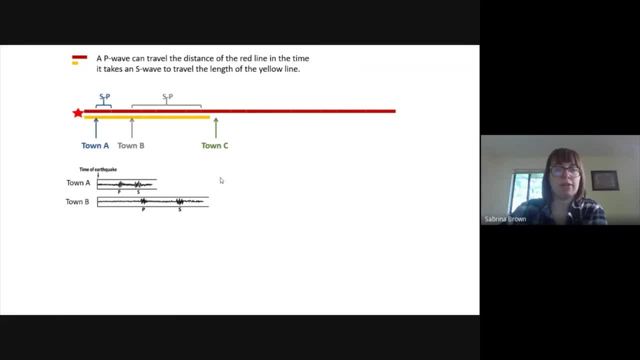 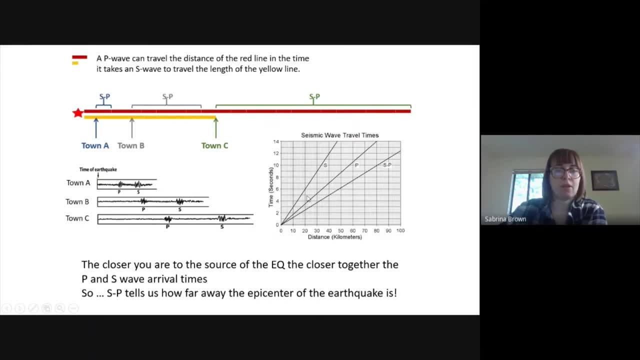 And then, if we keep going for town C, you can see how that distance keeps getting larger and larger. All right to the source of the earthquake, the closer together the p and s wave arrival times will be and because of that, the the difference between when the p wave and the s wave arrives that sp. 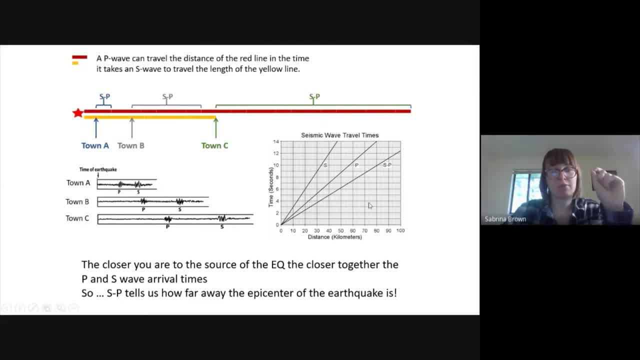 interval can tell us how far away the epicenter of the earthquake is, which is really cool, and so we can use diagrams like this one and using: uh okay, we know that it took, let's say, 10 seconds. um, we have an interval of 10 seconds between when our p wave arrived and when our s wave arrived. 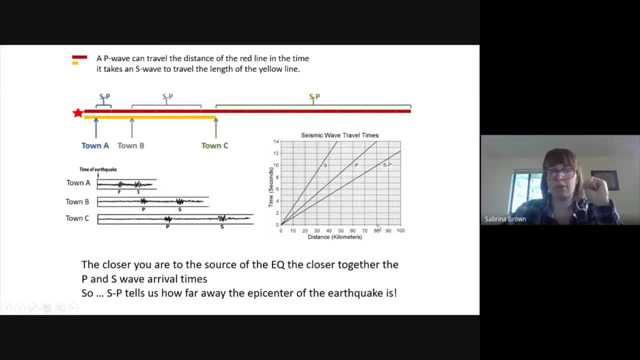 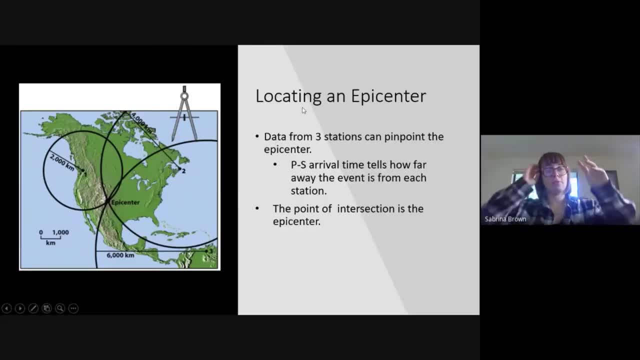 at on our seismograph so we know that the epicenter was 80 kilometers away, all right, so we can tell how far away an earthquake's epicenter was using one seismogram. so if we have three seismograph um data, right, if we have data from three seismographs or three stations, we can. 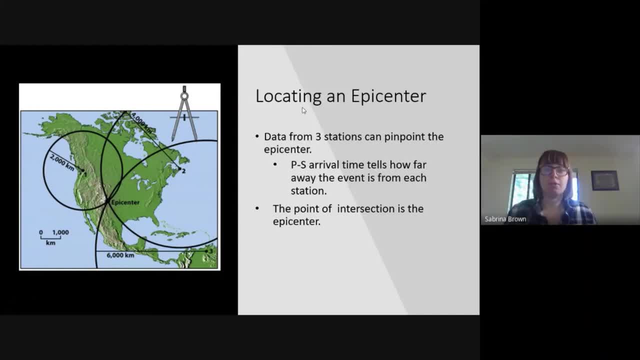 pinpoint where the epicenter actually was, because we can use um you know, trigonometry, which you know is like something i never thought i'd use again in my life until i started um doing science in college. and so again, remember that sp arrival time tells you how far away each of the events is. 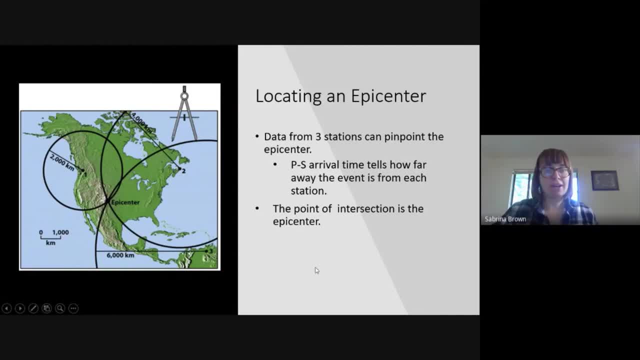 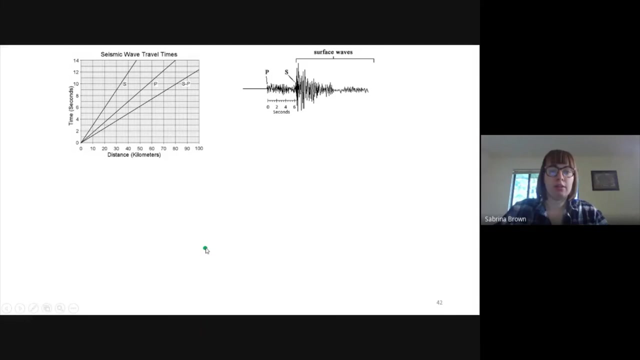 from the each of the stations. so if we use that as the radius of a circle, we can draw a circle around the station, find where those three circles intersect, to locate the epicenter of the earthquake. so here, for example, we have uh station, one which we have as green here it has an sp. 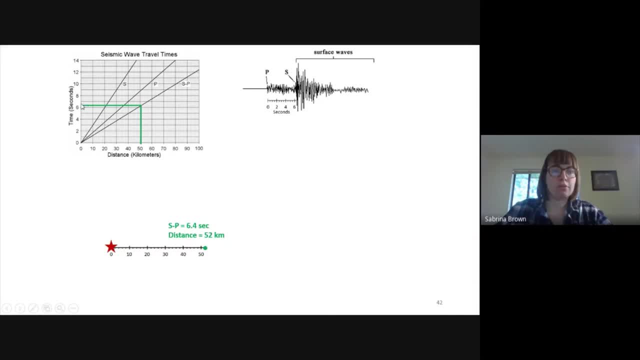 interval of 6.4 seconds and if we use this diagram with the sp interval of 6.4, we get a distance of 52 kilometers. so we know that the epicenter- epicenter is 52 kilometers away from that station, but we don't know what direction that epicenter is away from the station. it could be in any direction. 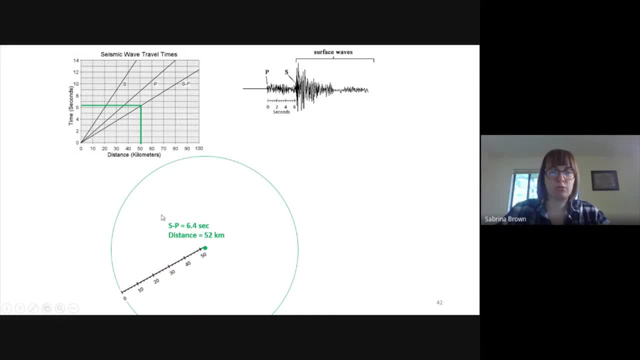 so we draw a circle around our station with a radius of 52 kilometers. right, so the station, the epicenter, could have occurred within 52 kilometers in any direction of the station. okay, so we have the second station, which is yellow, with an sp interval of 7.4 which, if we use our seismic wave travel time diagram, we see.